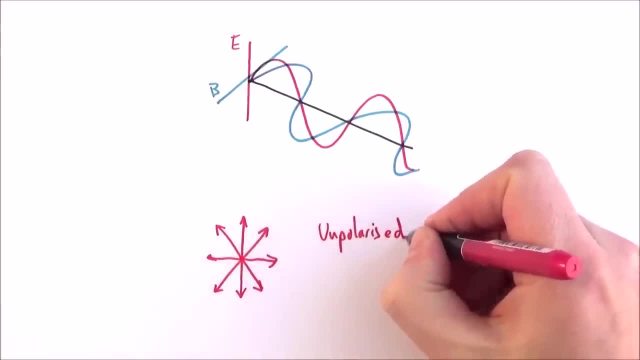 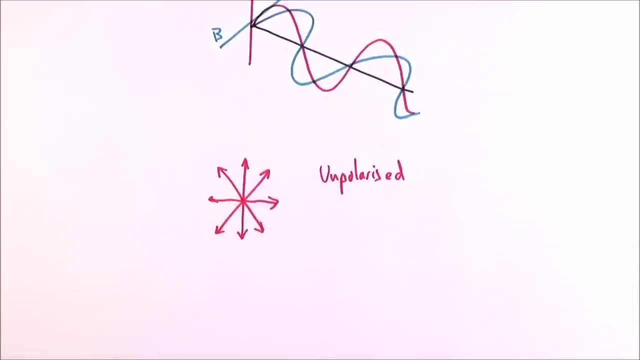 this is like the light maybe emitted from a lightbulb, or maybe the sun, And what we can do is we can apply a filter to this and what we can start to do is filter out some of those vibrations. So if we had a filter that only had a slit that was vertical, what? 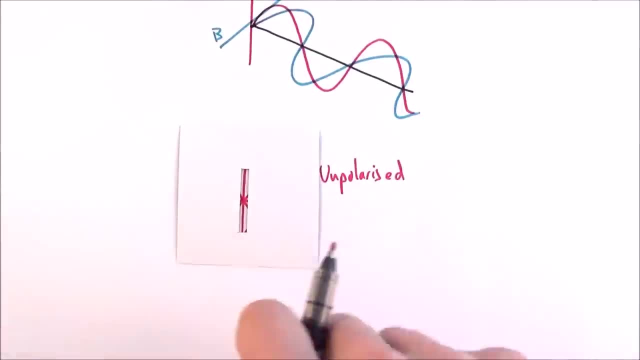 that would do. that would filter out all of the crossways and any light that's coming out at an angle, And what we'd have then is light that looks like this, And what we can then say is that light is plane polarised because it's been polarised into one plane. 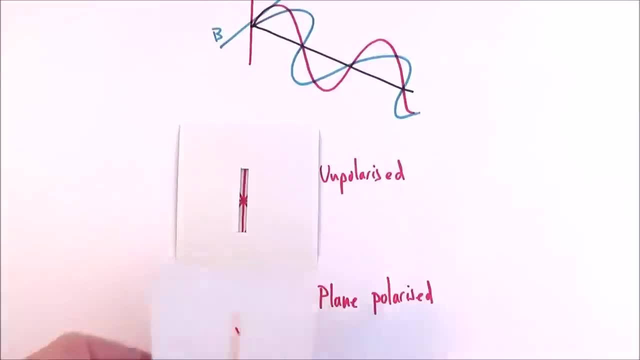 If we were to apply another filter to this, then again, all that light would get through if the two filters are in exactly the same plane. If, however, we rotate it, what we find is that the intensity of light that gets through decreases, And if we have two filters, that 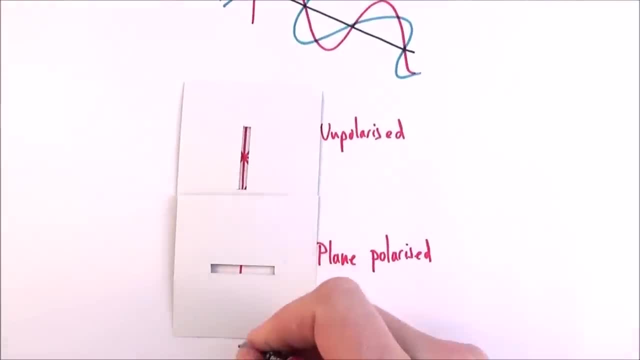 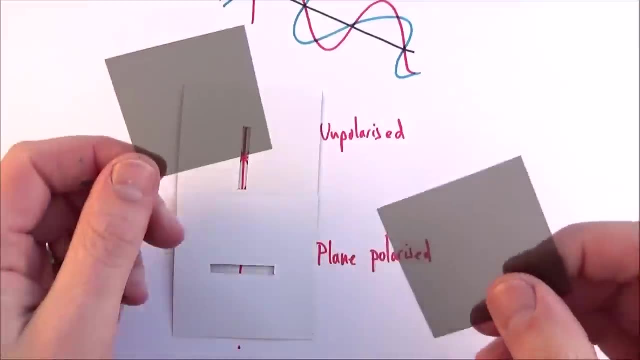 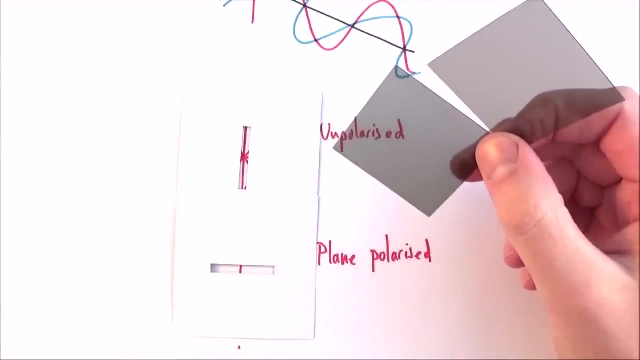 are at 90 degrees to one another. what we find actually is that none of the light gets through, And this blocks out the light completely. So we can do the same. We can use a couple of pieces of Polaroid. It's basically nitrocellulose And they're basically small crystals of quinine. 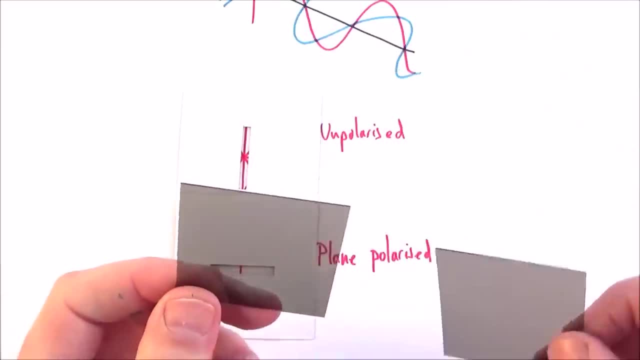 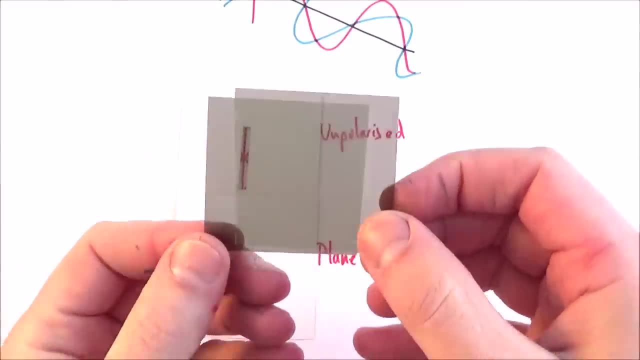 iodosulphate. Yeah, I did have to look that up. But what they do is when they absorb light, they only emit light, that is, plane, polarised. And if we have the two filters, which are perfectly in line, so both vertically, it lets some of the light through, But actually it only. 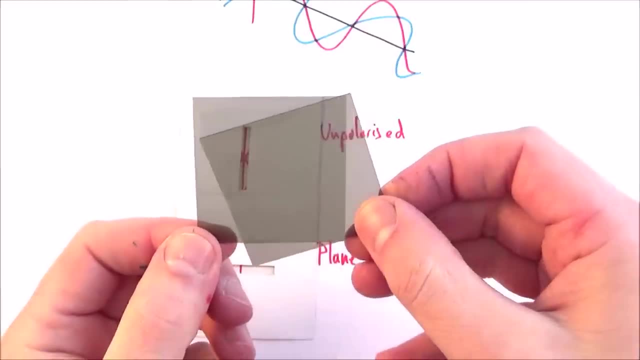 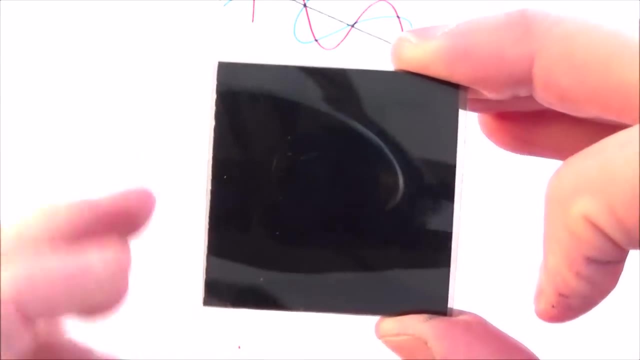 lets about 50% of that light through. As I start to rotate it, I can see that the light is coming through, So what I can do is I can rotate them. We can see that less and less light gets through until eventually, if we have the two filters at 90 degrees to one another, none of that light gets through. 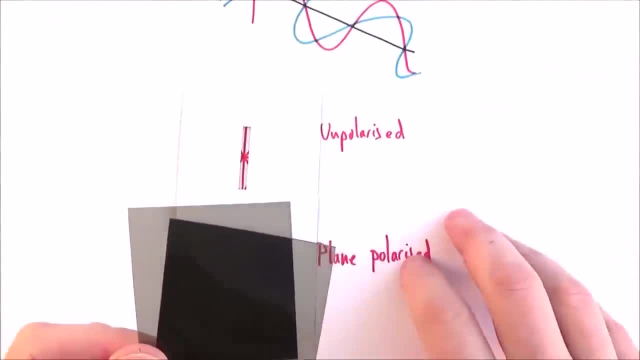 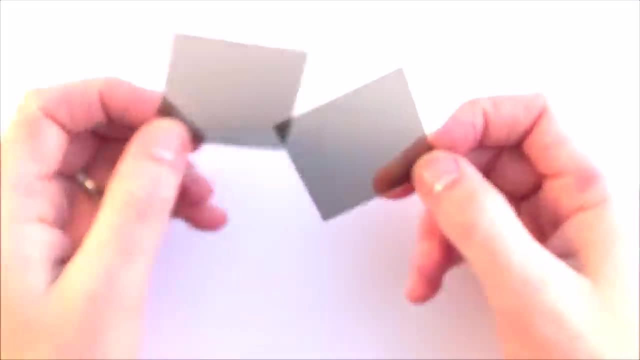 And what we have. there is just an example of how we can polarise light. So we can use a light meter to have a look at the intensity of light that goes through a couple of filters. So we've got a filter to make the light plane polarised, And then 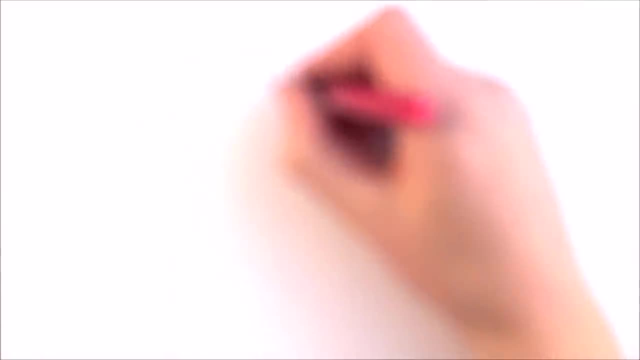 we have the analyser And actually what we find is that the amplitude of the light that comes through is equal to the original amplitude of the light that came out of that first filter times, cos theta. However, we already know that the intensity of light is proportional. 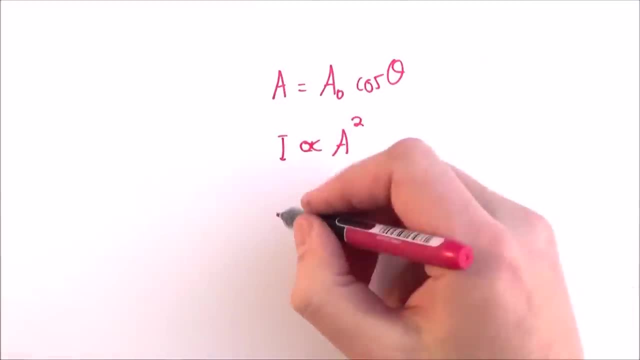 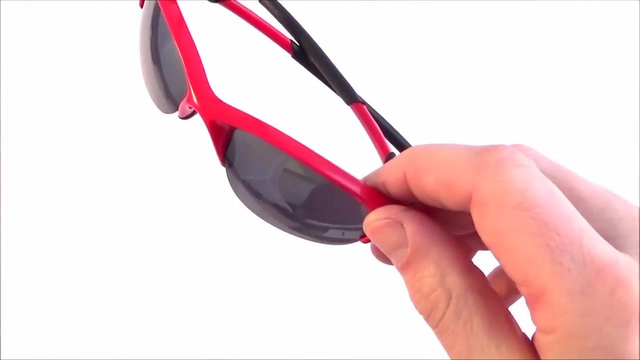 to the amplitude squared, And that was in a previous video. So we can then say that the intensity of the light transmitted through the analyser is equal to the original intensity times, cos squared, theta, And this is known as Maillis's law. Why is this important? Well, we have Polaroid sunglasses, And what these do is these cut. 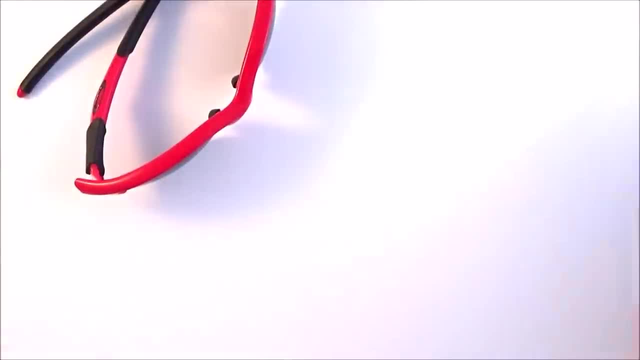 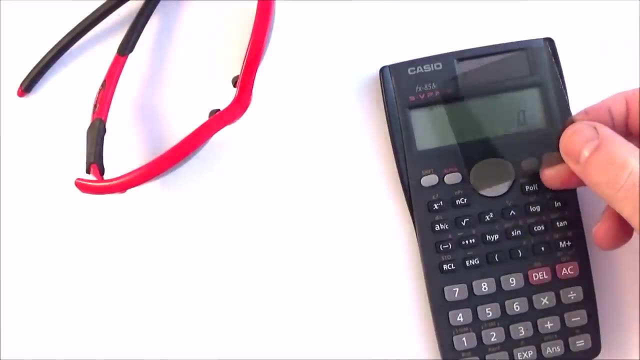 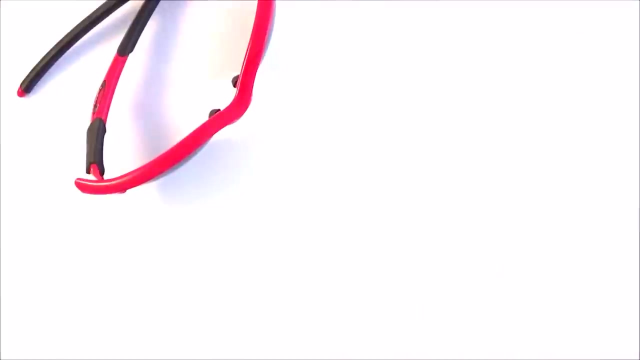 down on the glare from reflected light. Also, the light emitted by many laptops and screens and things like calculators is also polarised, which I can show maybe with that filter As I move that filter. it basically filters out that plane polarised light And reflected. 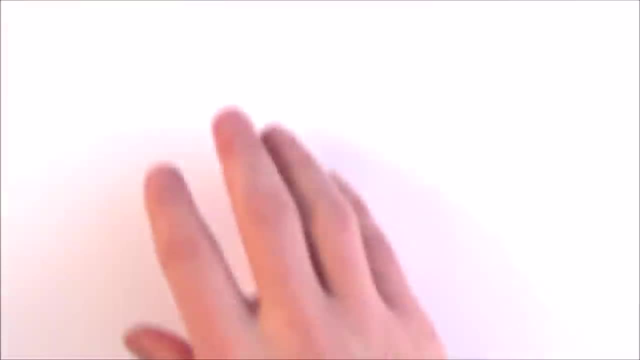 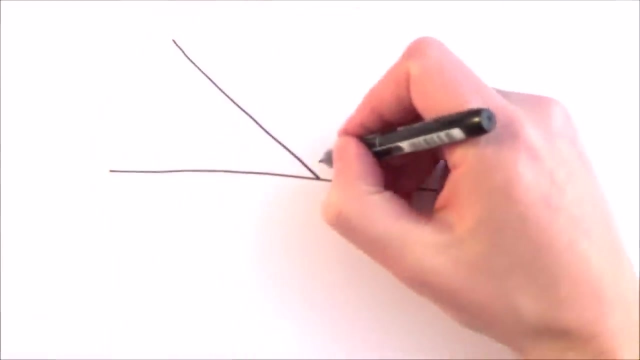 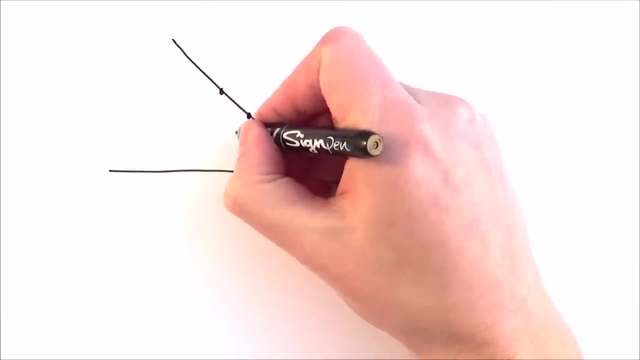 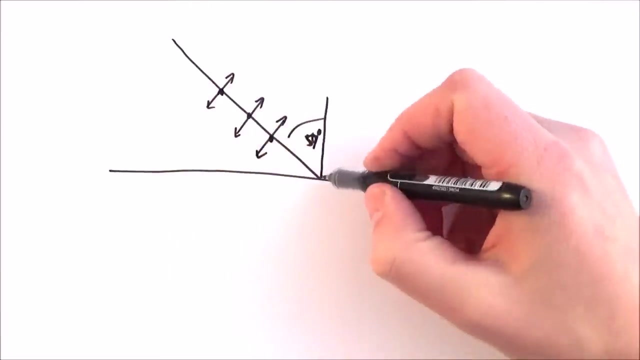 light from water is something else, which, again, that's what the sunglasses cut down on. If we look at some water and there's light that comes in at a certain angle- if the angle is about 57 degrees- then the light that comes in is unpolarised As it hits the surface. 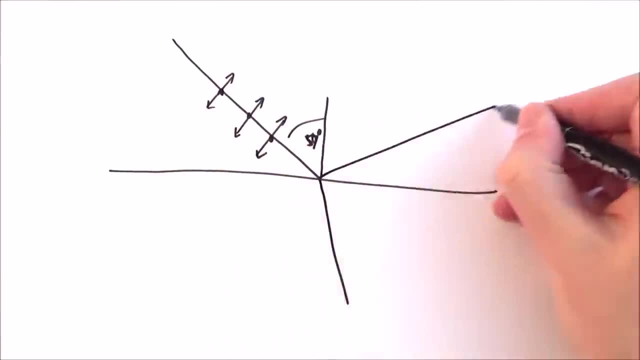 some of the light is refracted down and some of the light is reflected, And what we find is that the light reflected down is still kind of reflected. It's still kind of unpolarised, But all the light that's reflected is plane polarised. 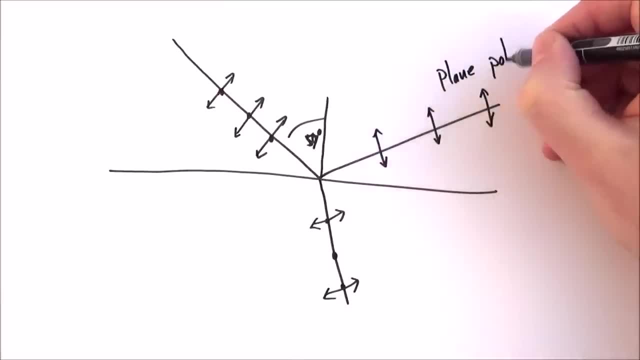 So this is plane polarised light And you can often see the effect if you look at windows. or perhaps if you're driving and you see a low winter sun on a wet road, you really kind of have that glare And we can really cut that down by looking through the plane polarised. 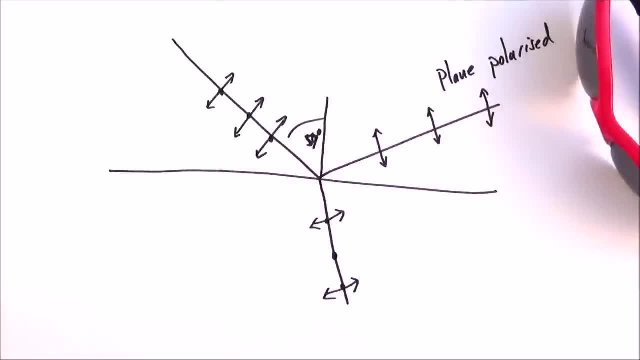 light with the polarised sunglasses, And what this has the effect of doing is effectively blocking out all of that reflected light, So you can actually see the road a lot more clearly. A final example is if we have two polaroid filters that are at 90 degrees to one another. 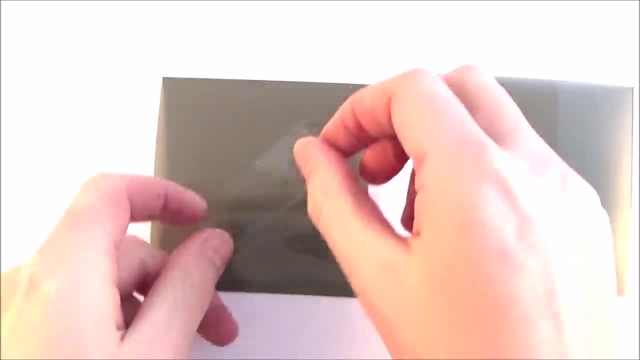 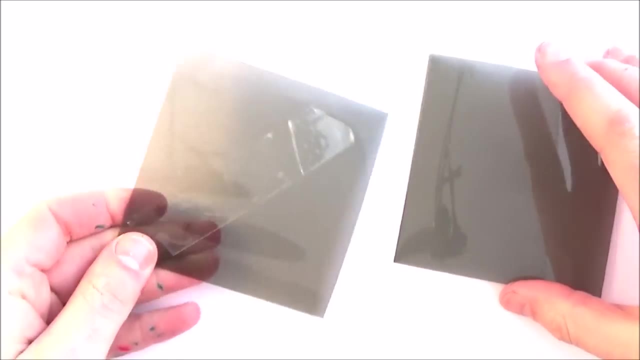 and between the two filters we put in a piece of tape. Although in real life you might have a model of an engineering component, perhaps part of a hook or a bridge- is when you put them back over each other we can actually look at stresses in that material And this: 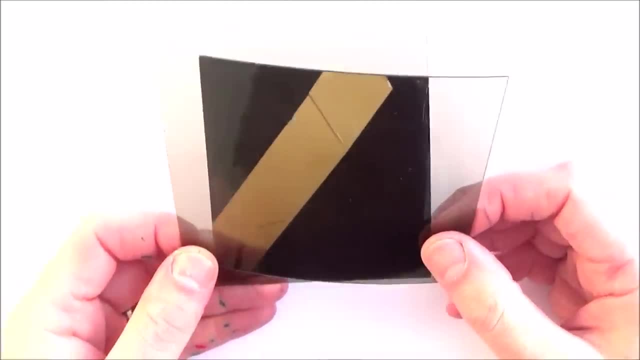 is a really useful way of analysing shapes. A bit of stress analysis.